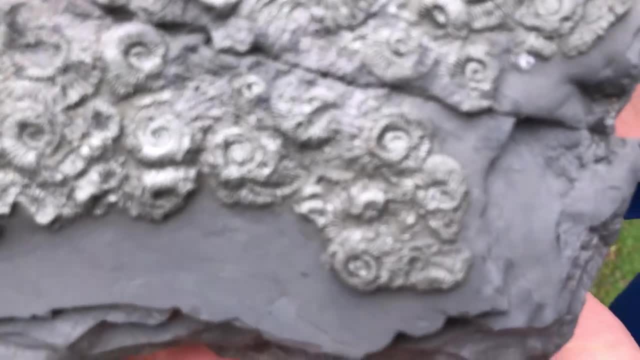 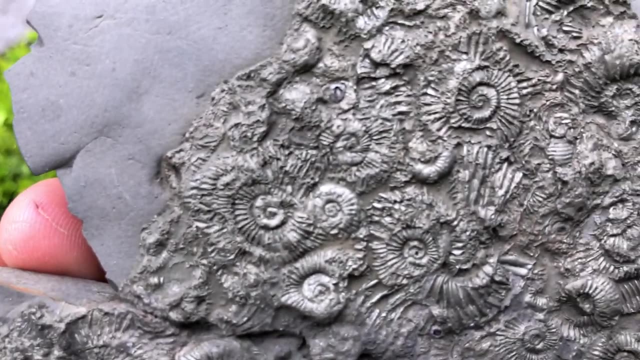 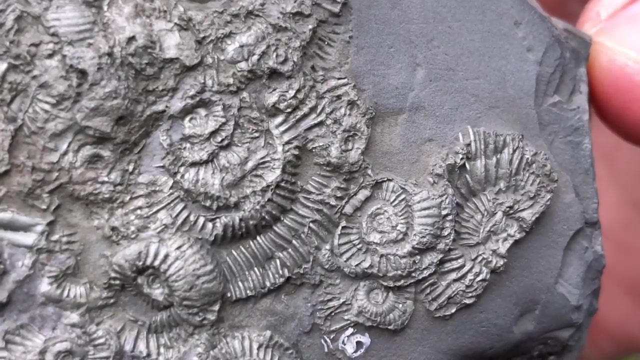 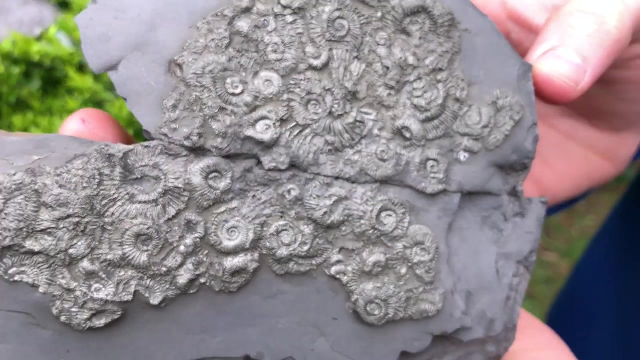 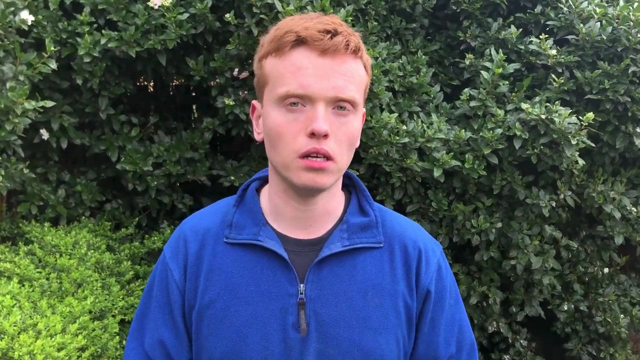 i've also got one here. so many ammonites- i've not counted how many there are, but as you can tell, it's an absolute abundance. the next thing for us to do now is to glue together the shale pieces we looked at earlier with the crinoid in. then, once it's glued together, we'll be able to start making some. 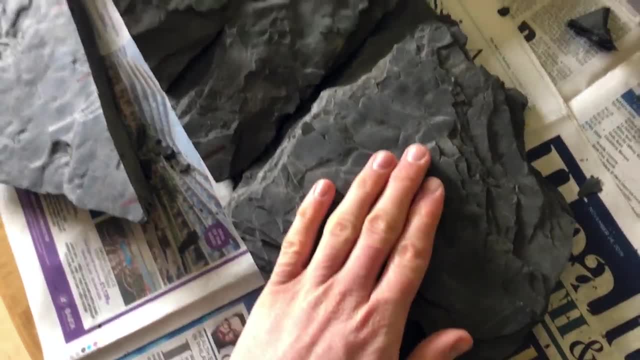 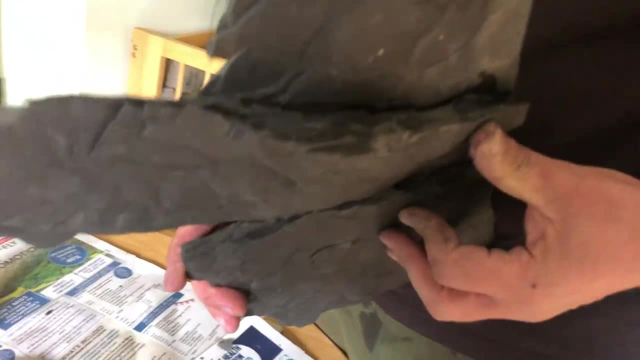 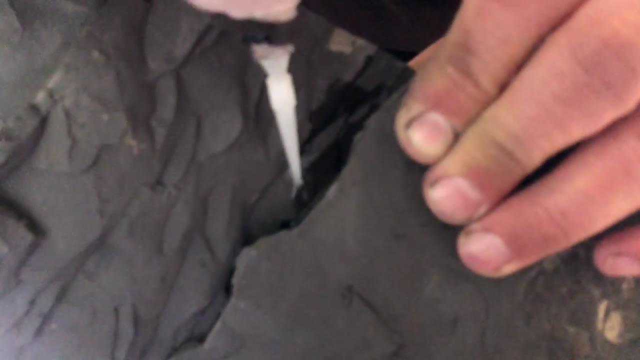 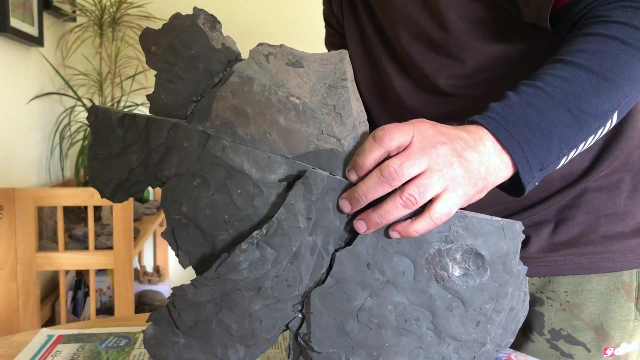 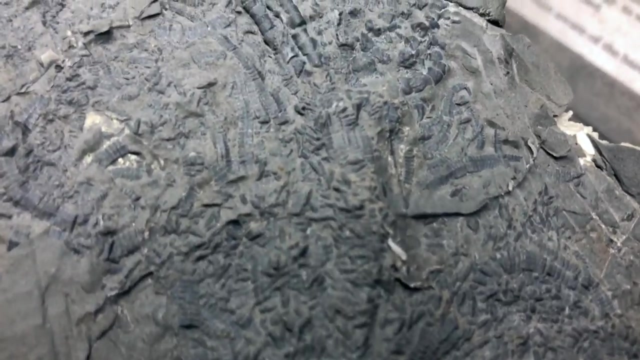 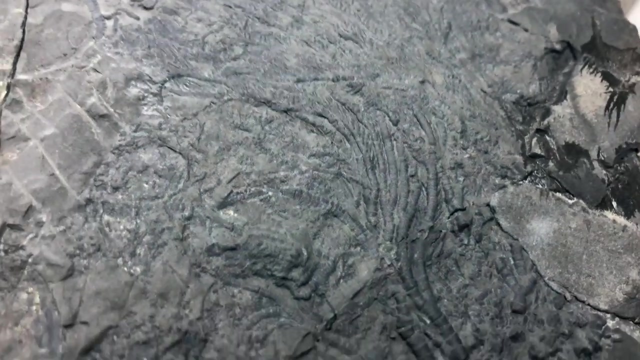 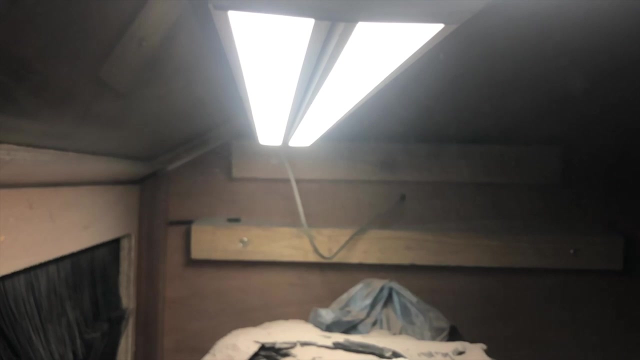 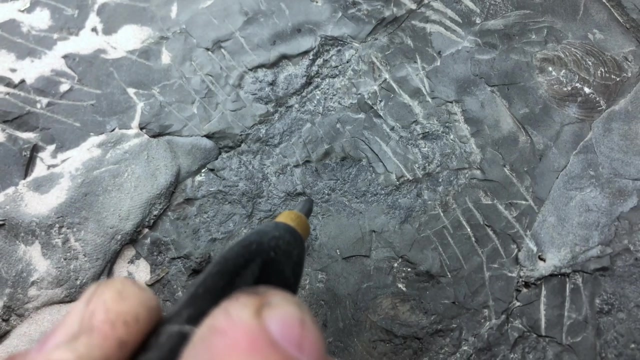 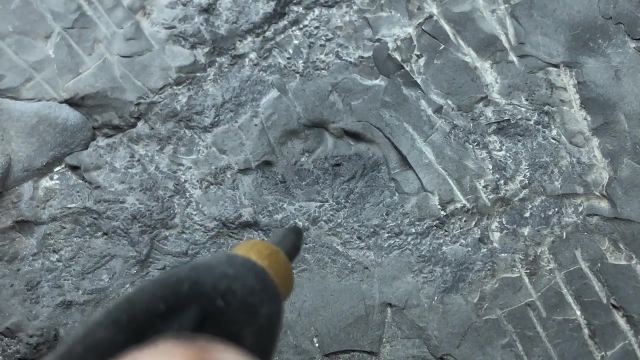 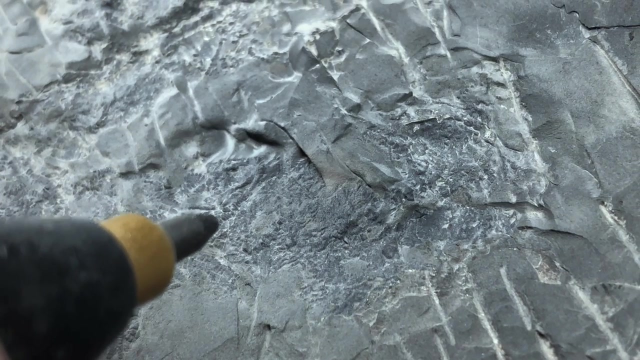 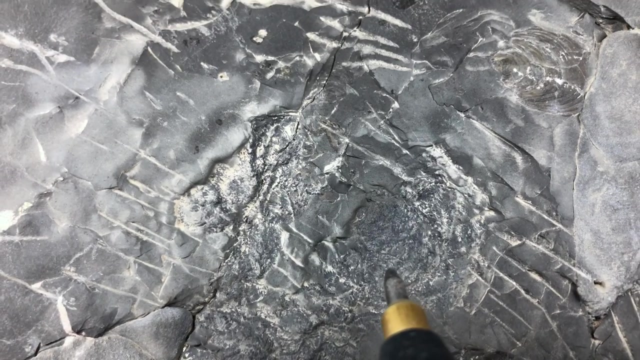 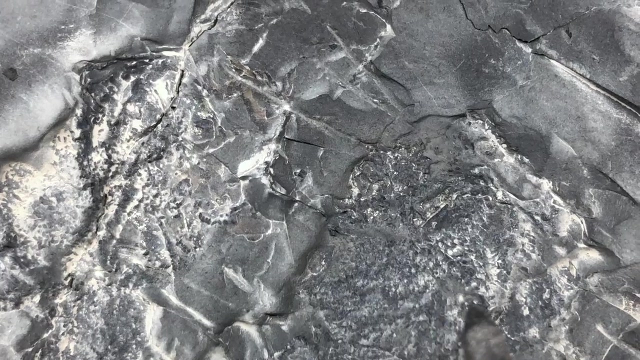 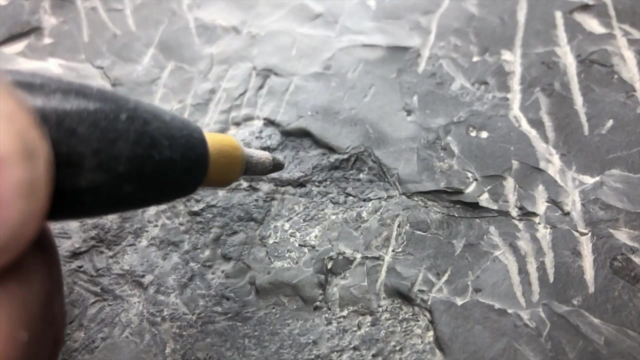 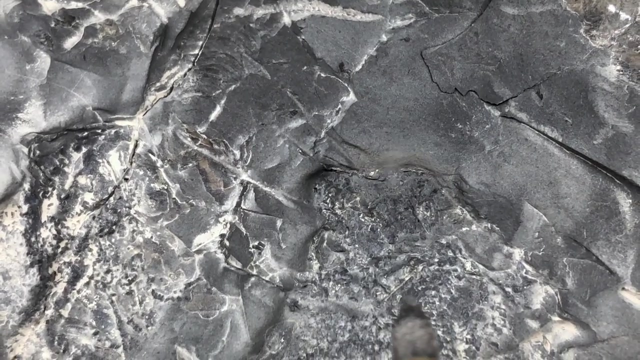 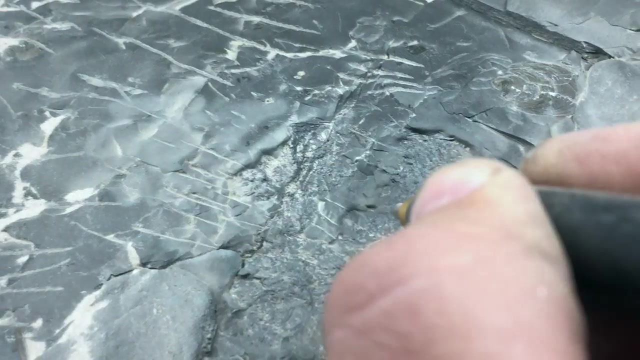 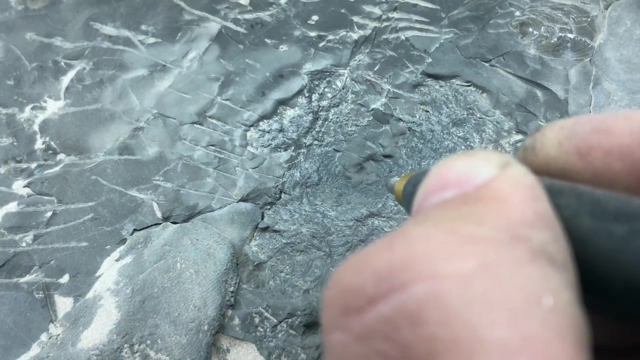 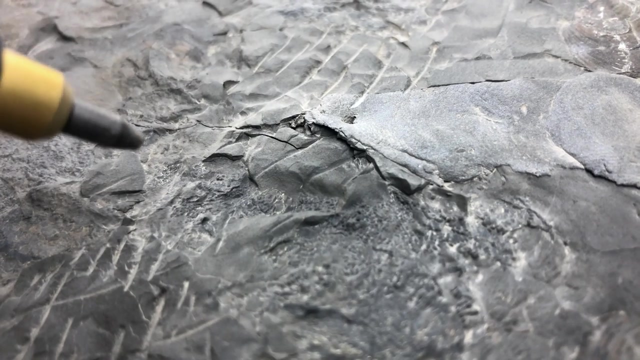 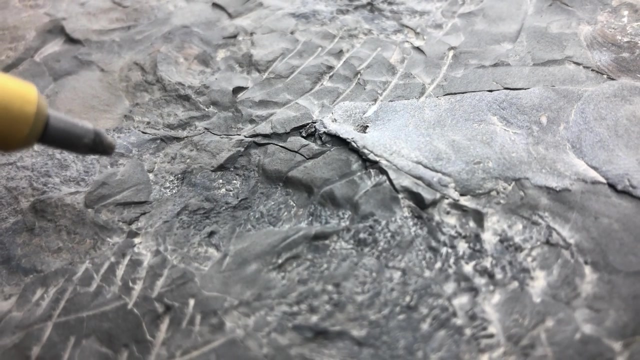 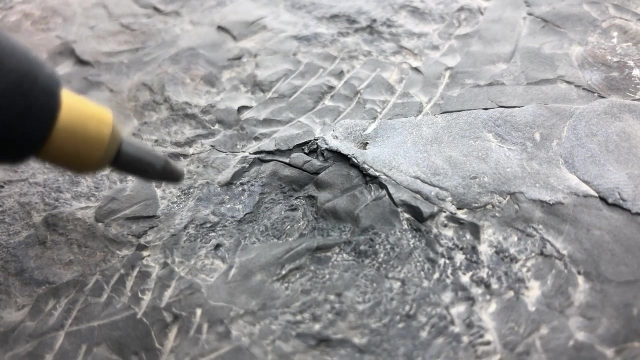 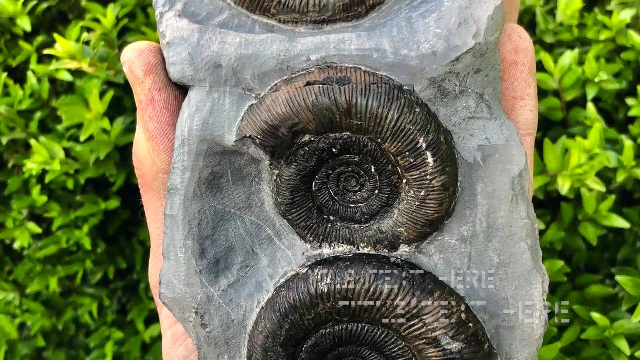 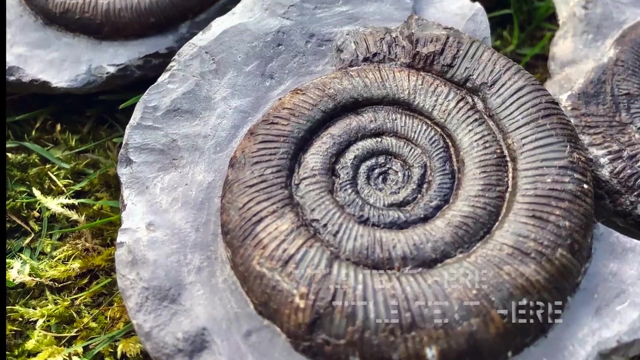 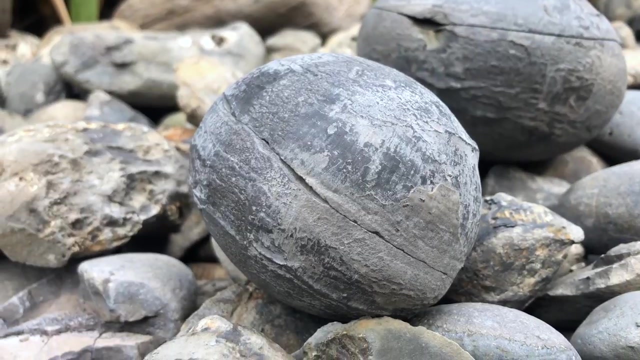 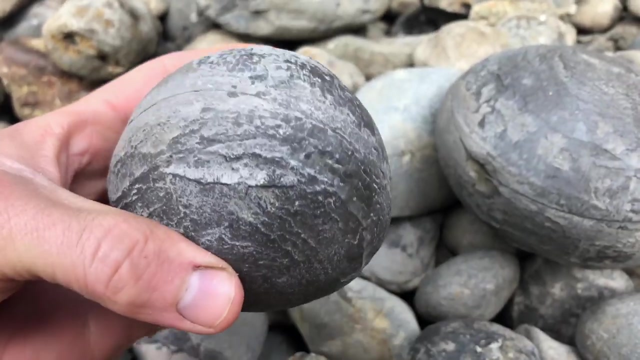 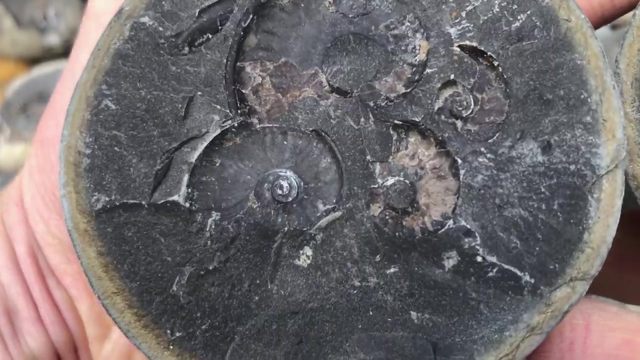 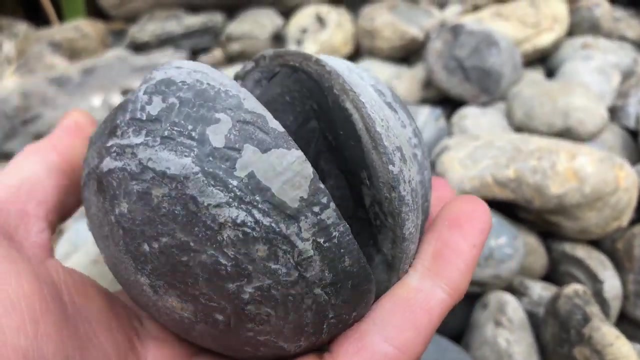 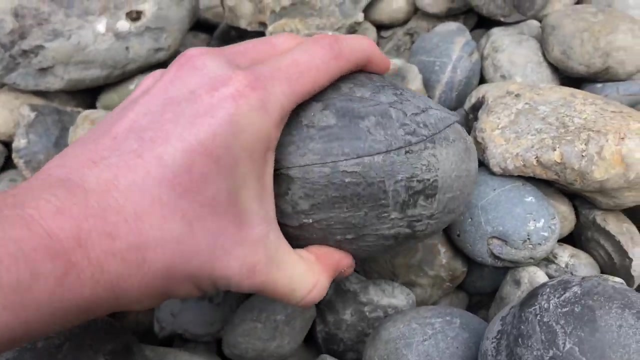 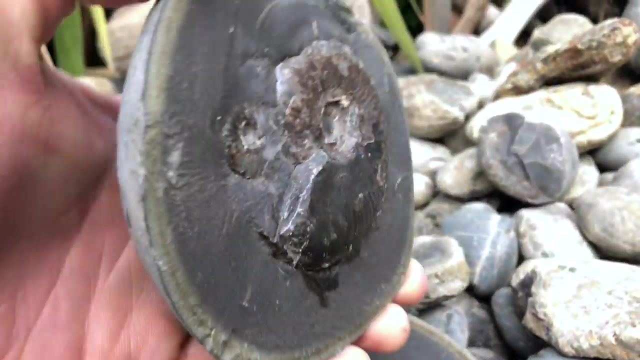 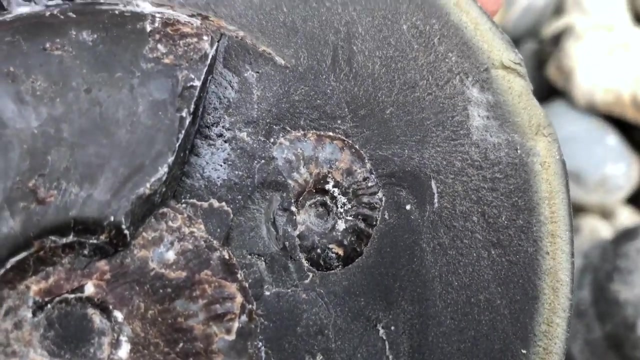 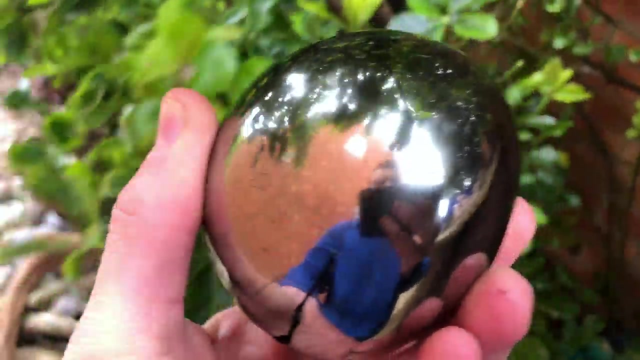 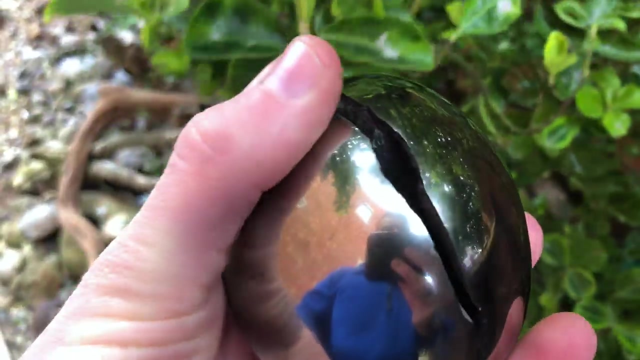 progress on the preparation. just started piecing it together. quite difficult to make it all glued together and it's just pretty straight edges, so so, so, so, so it's absolutely beautiful, like a golden mirror. next thing to do is to prepare the ammonites on the inside. 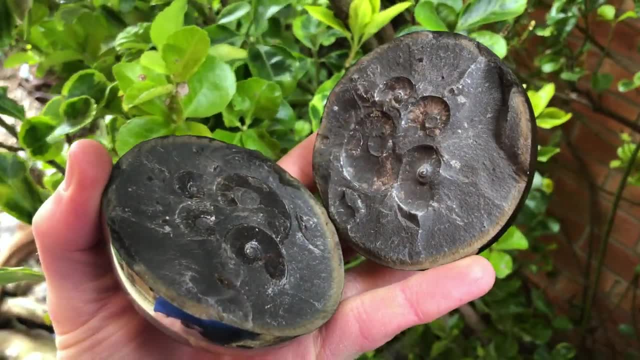 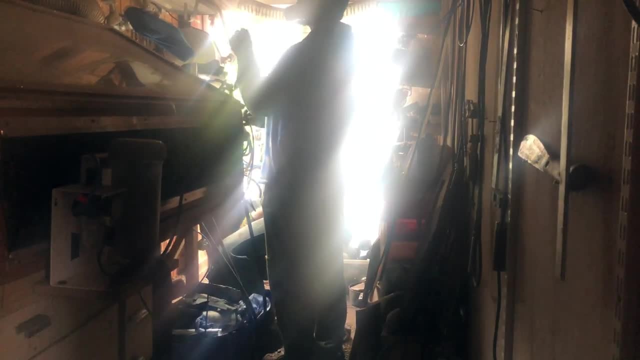 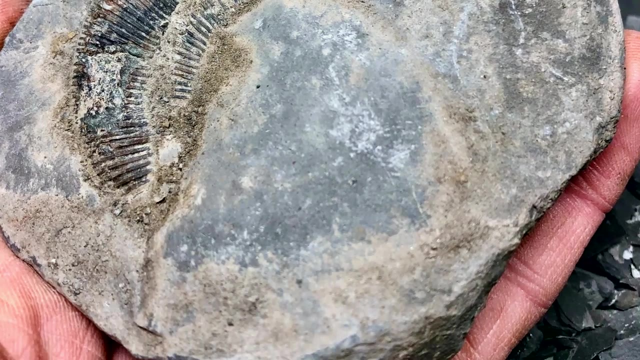 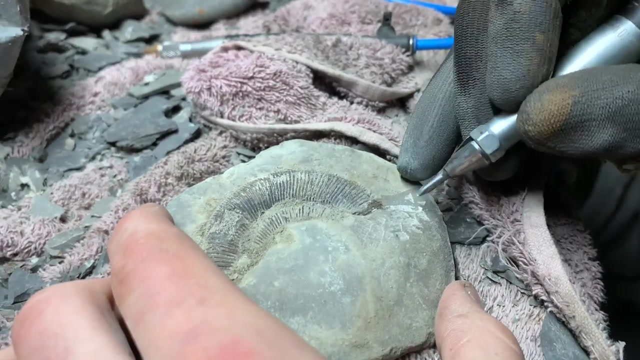 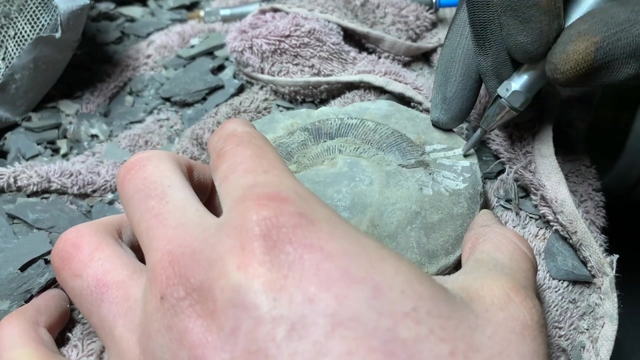 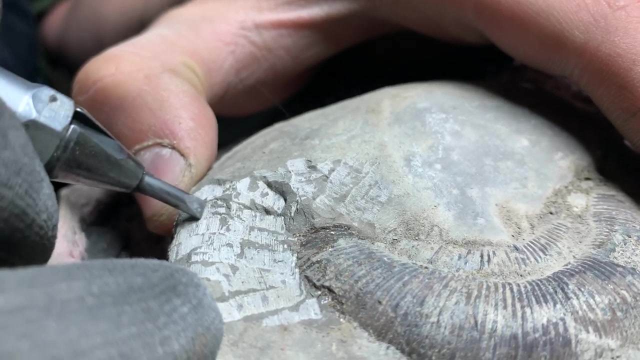 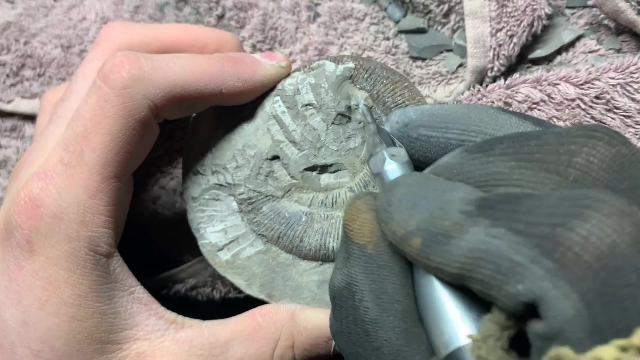 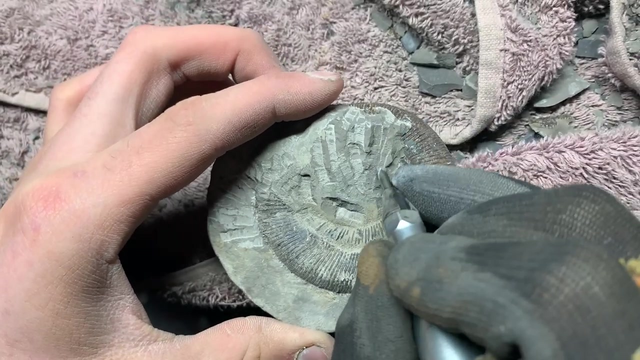 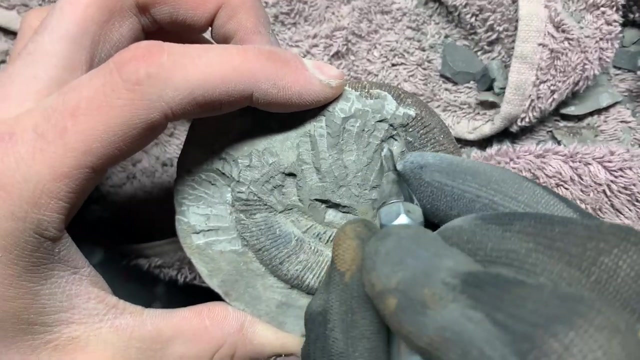 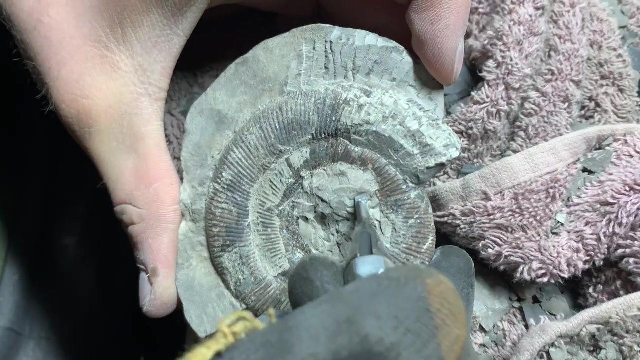 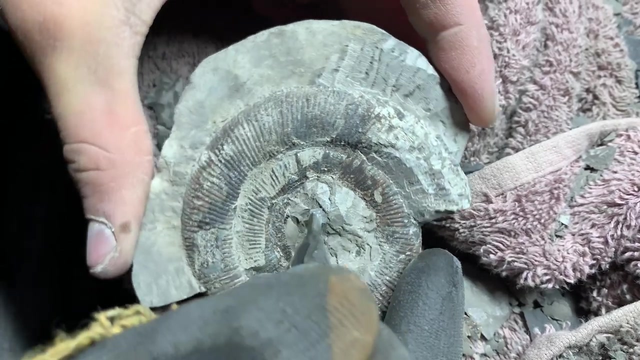 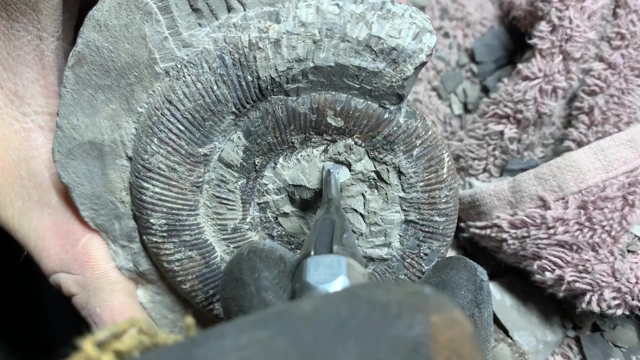 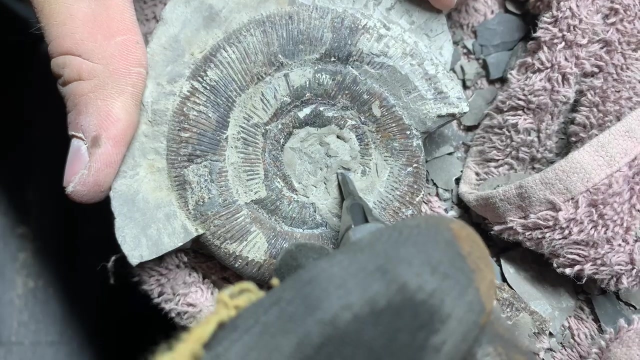 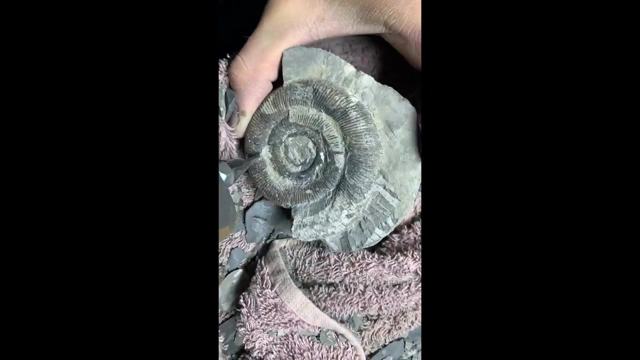 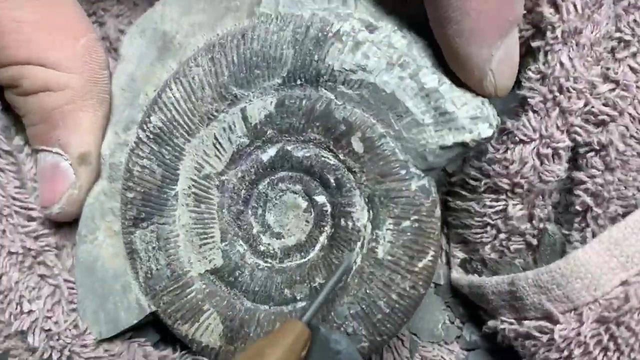 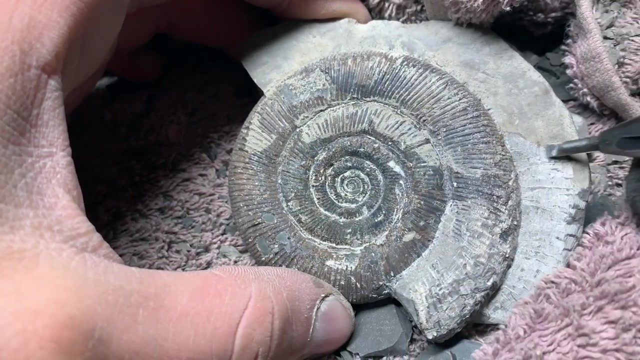 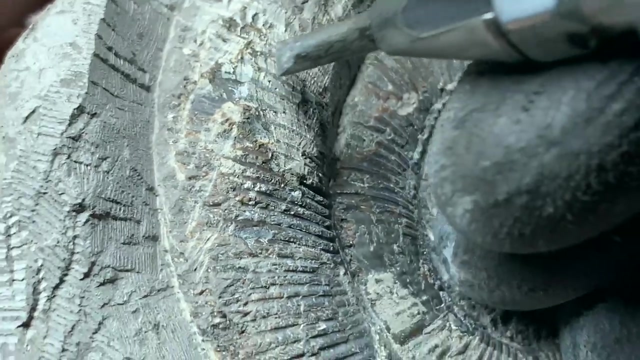 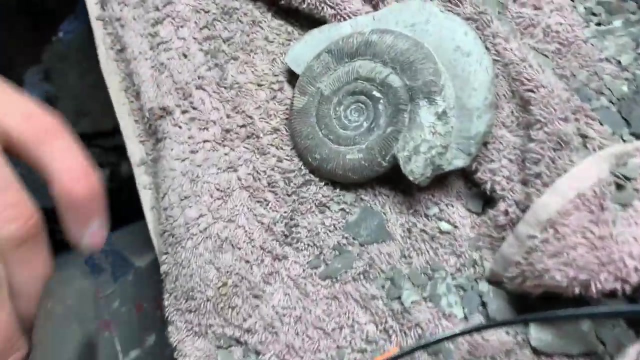 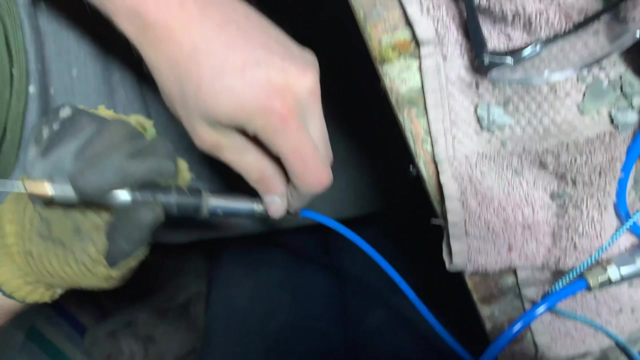 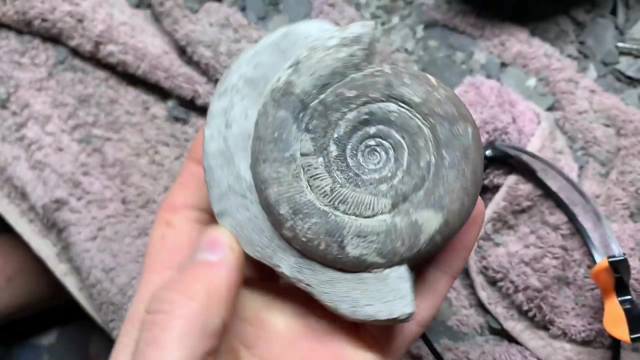 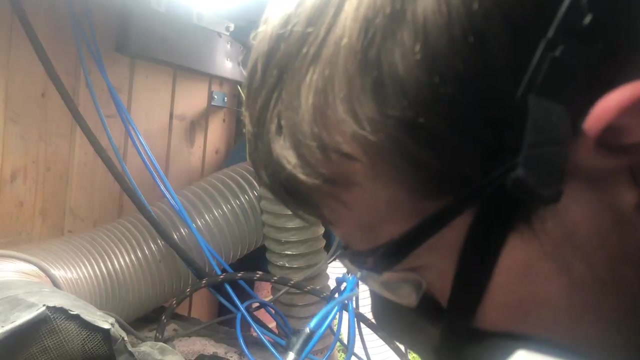 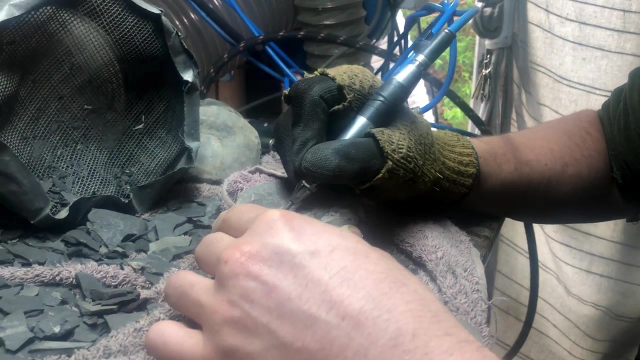 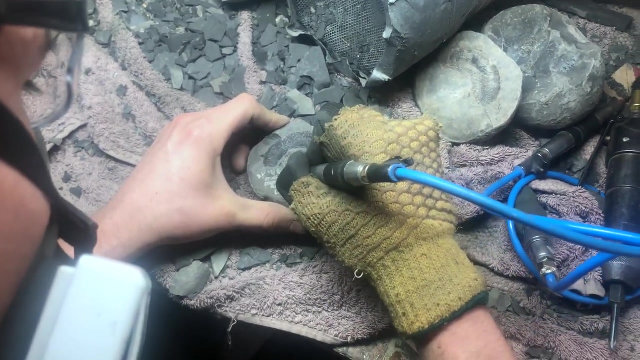 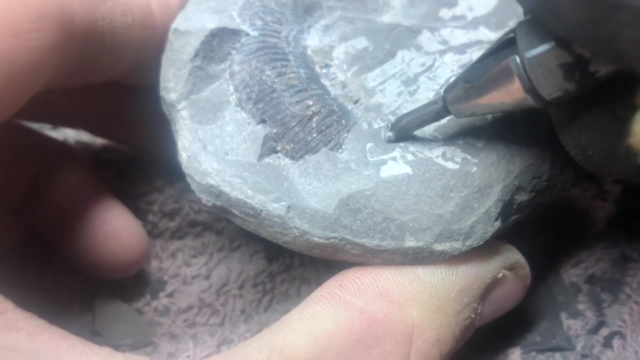 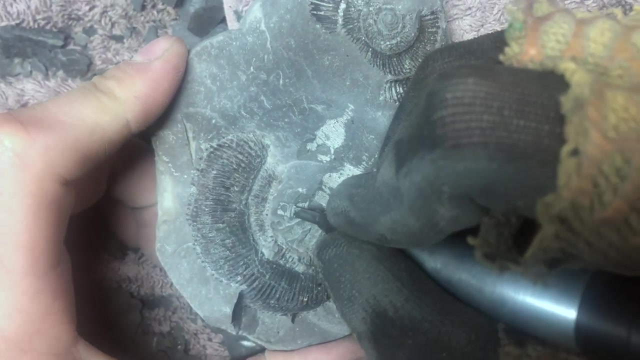 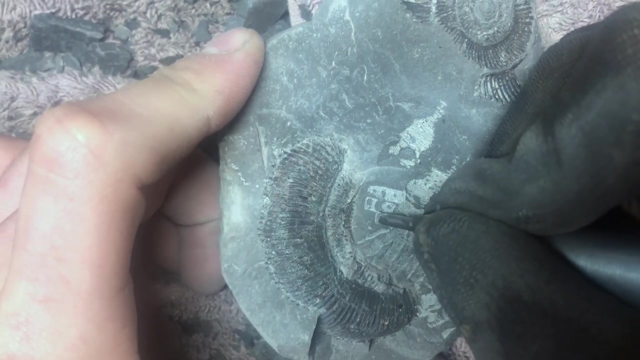 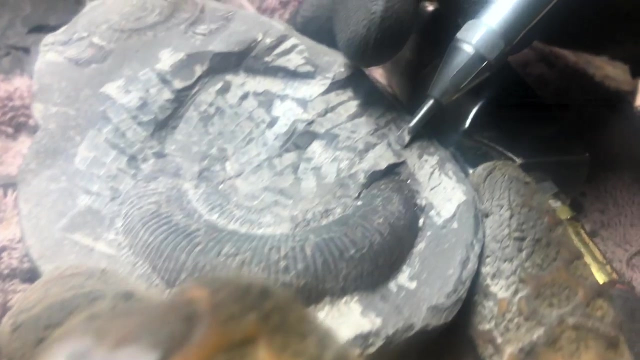 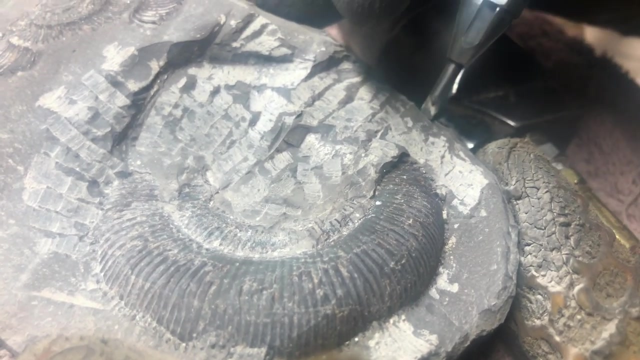 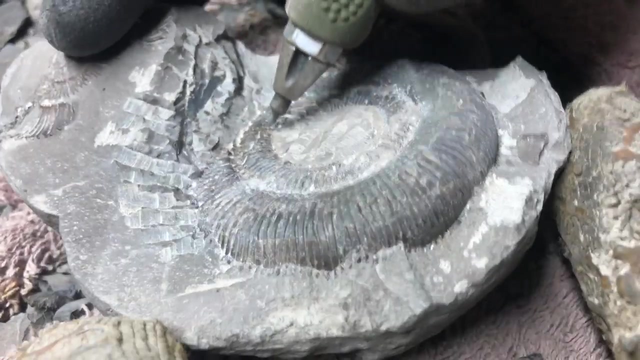 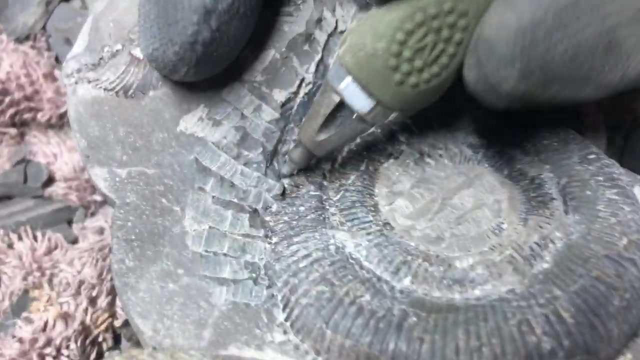 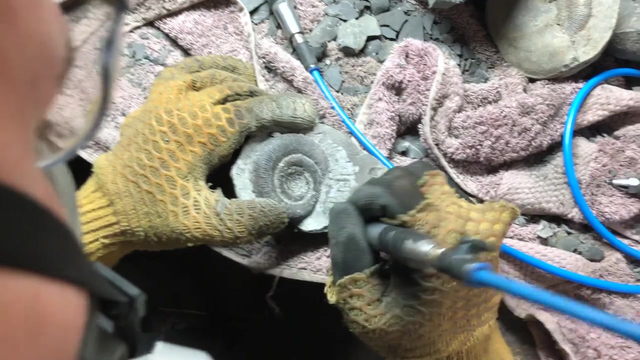 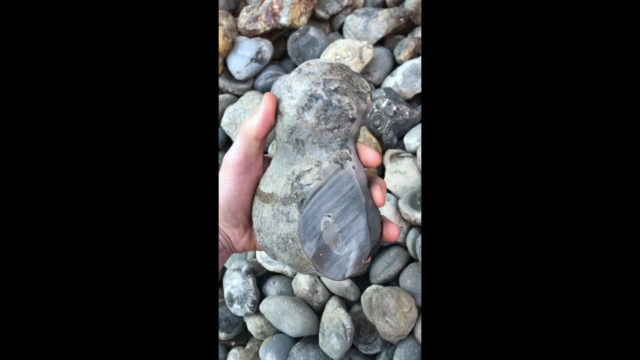 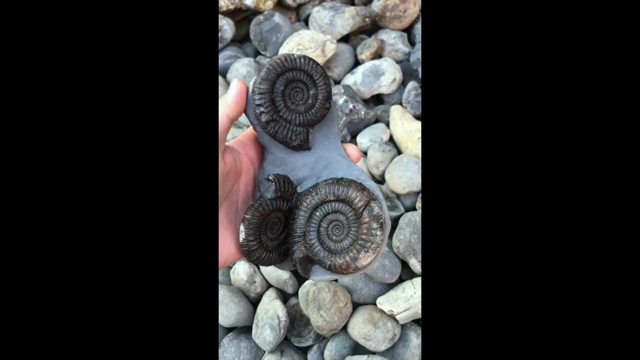 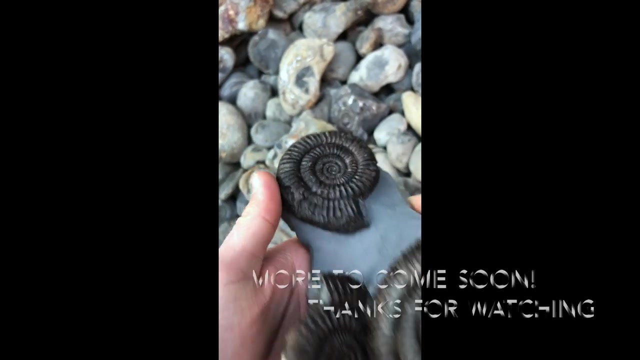